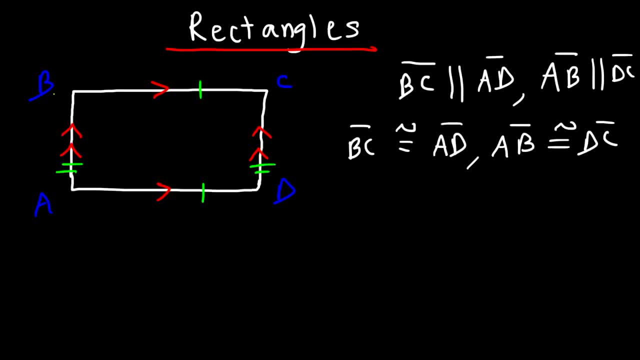 Now, all of these rectangles are congruent. Now, all of these rectangles are congruent. All angles are right angles. They're all equal to 90 degrees. So, angle A, angle B, angle C, angle D, they equal 90.. Now the next thing you need to know are the diagonals. The diagonals. 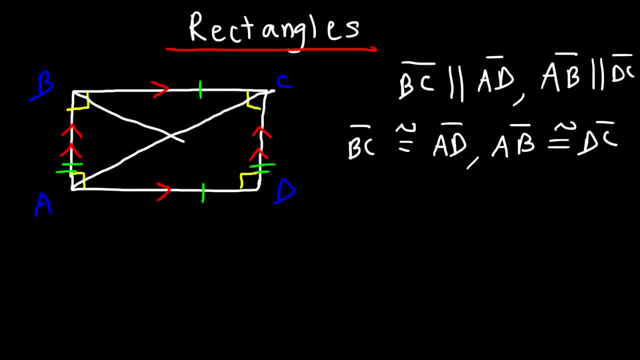 are congruent to each other. So diagonal AC is congruent to diagonal BD. Now also the diagonals bisect each other. So what that means is that AE is congruent to EC and BE is congruent to ED. So we can write it like this: AE and EC are congruent and BE is congruent to ED. 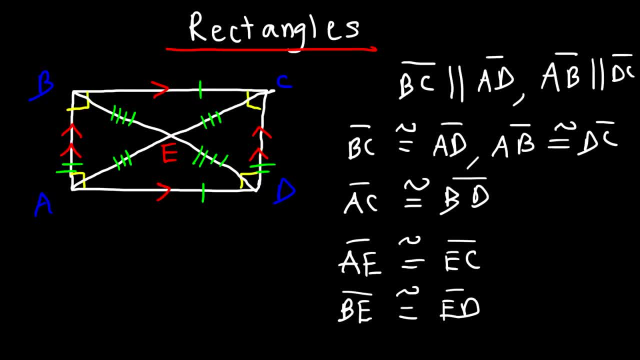 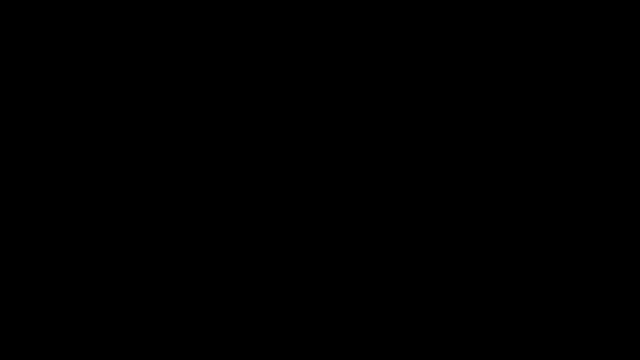 which makes E the midpoint of AC, And E is also the midpoint of AC, So that's the quadrilateral of the diagonal, And E is also the midpoint of AC, And so you need to know the coordinates of the angles. So this is our left and right angles. So 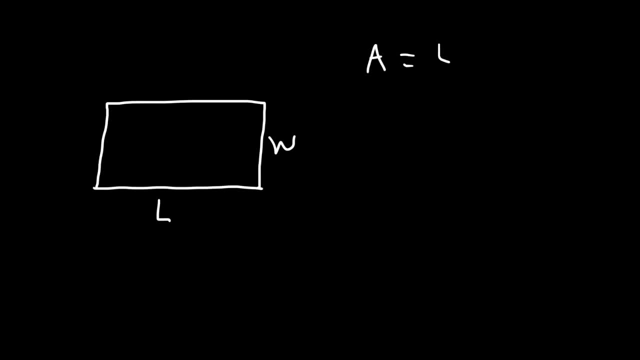 this is the area we need to know. So here we have the length and the width of the rectangle. So let's say we have the width of the rectangle And we need to calculate this with the diagonal. Now we want to scale this diagonal to see if we can have the potential of the diagonal. 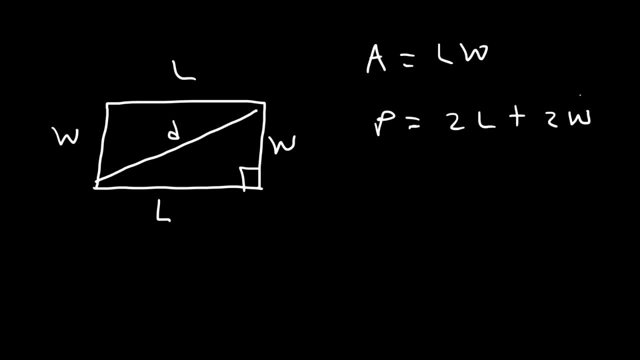 to be the same as the width of the rectangle. So the primary theorem for a triangle is this: LE. This is the formula for the diagonal. So let's say this is the left and the width of the rectangle. The area is the length times the width. The perimeter is the sum of all four sides, so it's 2L plus 2W. 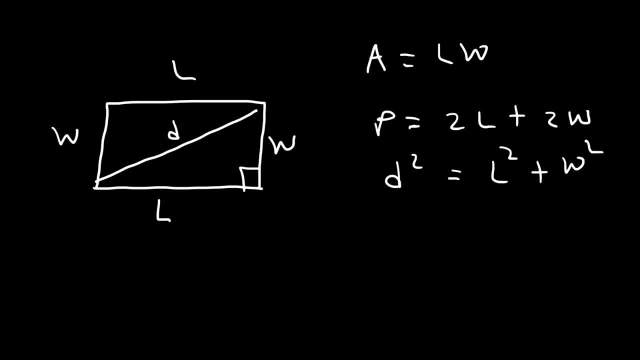 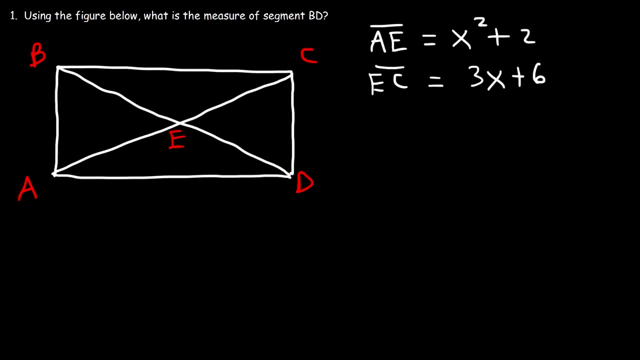 d squared is l squared plus w squared, so you can use that to calculate the length of the diagonal. now let's work on some example problems. our goal is to determine the measure of segment bd and we're given ae and ec. so how can we do so? but we know that the diagonals bisect each other. 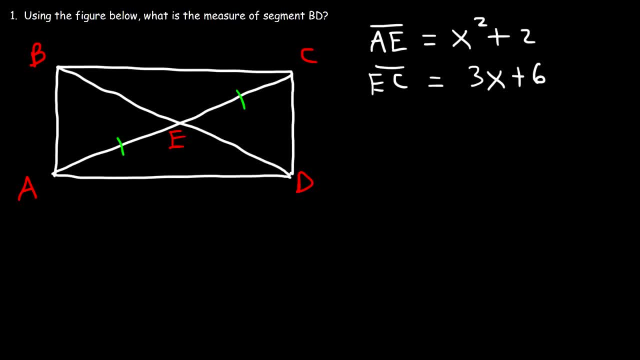 so e is the midpoint of ac, which means that ae and ec- they're equal to each other. so if we set them equal to each other, we could say that x squared plus 2 is equal to 3x plus 6.. so i'm going to take everything from the right side and move it to the left side. 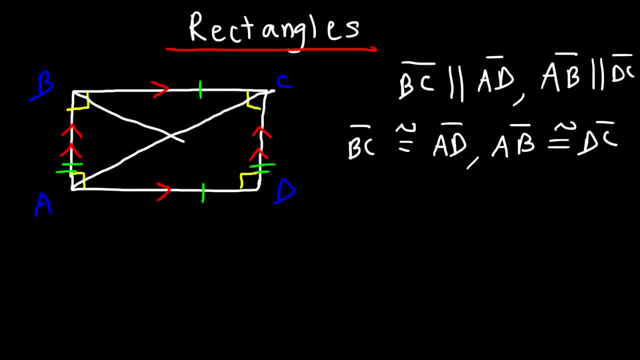 are congruent to each other. So diagonal AC is congruent to diagonal BD. Now also the diagonals bisect each other. So what that means is that AE is congruent to EC and BE is congruent to ED. So we can write it like this: AE and EC are congruent and BE is congruent to ED. 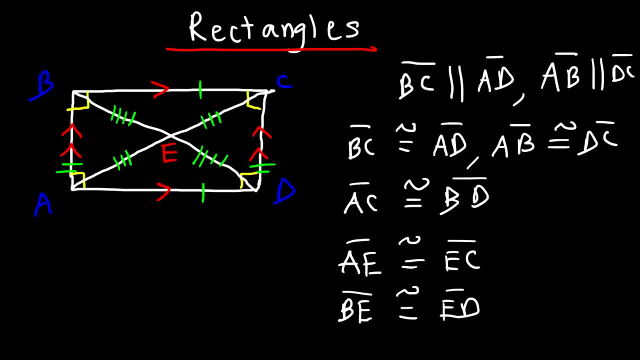 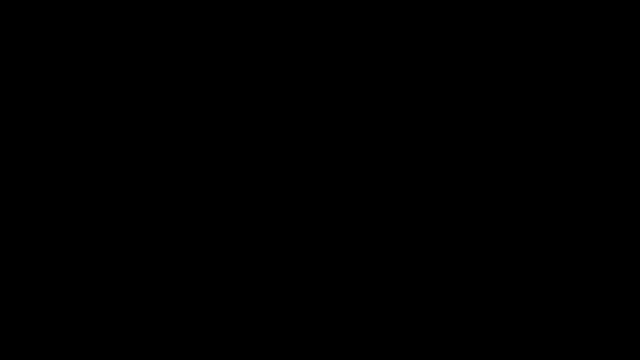 which makes E the midpoint of AC And E is also the midpoint of AC. So that means AD goes negative and d squared is L squared plus W squared, So you can use that to calculate the length of the diagonal. Now let's work on some example problems. Our goal is to determine the measure of segment BD. 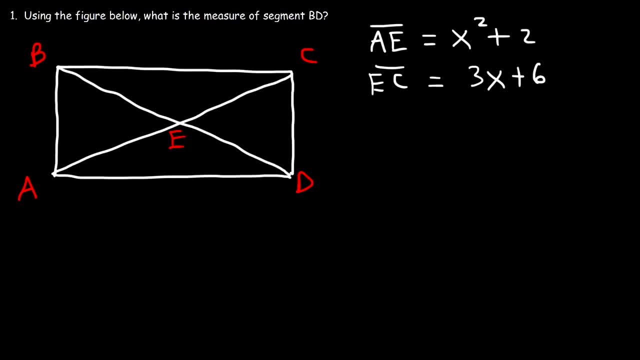 And we're given AE and EC. So how can we do so? But we know that the diagonals bisect each other. So E is the midpoint of AC, which means that AE and EC, they're equal to each other. So if we set them equal to each other, we could say that X squared plus 2 is equal to 3X plus 6.. 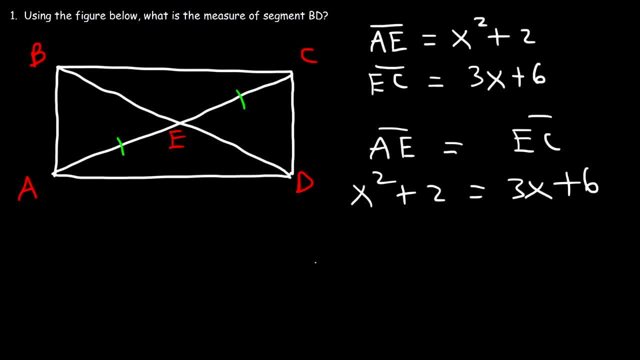 So I'm going to take everything from the right side and move it to the left side, So it's going to be X squared minus 3X plus 2 minus 6.. Now 2 minus 6 is negative 4.. And so we have a trinomial where the leading coefficient is 1.. 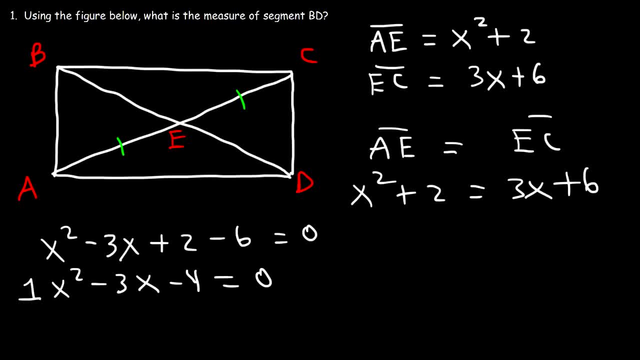 And we need to factor it in order to solve the quadratic equation. So what? two numbers multiply to the constant term, negative 4, but add up to the middle coefficient, negative 3? This is going to be negative 4 and positive 1.. Negative 4 plus 1 adds up to negative 3, and negative 4 times 1 is still negative 4.. 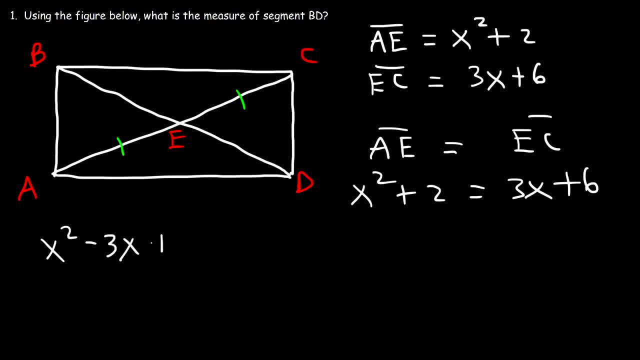 so it's going to be x squared minus 3x plus 2 minus 6.. now, 2 minus 6 is negative 4, and so we have a trinomial where the leading coefficient is 1 and we need to factor it in order to solve. 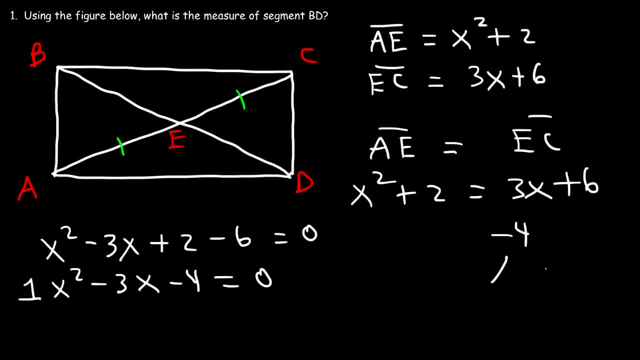 the quadratic equation. so what? two numbers multiply to the constant term negative 4, but add up to the middle coefficient negative 3.. this is going to be negative 4 and positive 1.. negative 4 plus 1 adds up to negative 3, and negative 4 times 1 is still negative 4.. so to factor, it's going to be x minus 4 times x plus 1. 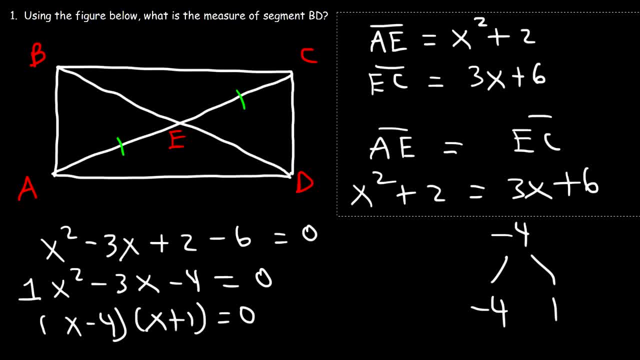 so now what we need to do is we need to set each factor equal to 3, so x minus 4 is equal to 0, so x minus 4 is equal to 0 and x plus 1 is equal to 0.. so x has to equal 4 and negative 1.. 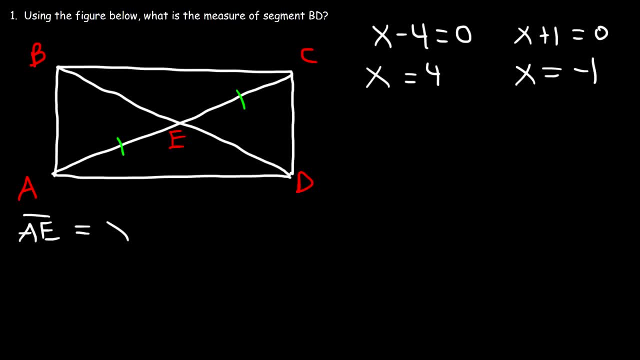 now let's keep in mind that ae is x squared plus 2.. because x is squared, we won't get a negative result for ae for using either of these two answers. now for ec, x is, i mean, ec is 3x plus 6.. so if we plug in negative 1, it will still give us a. 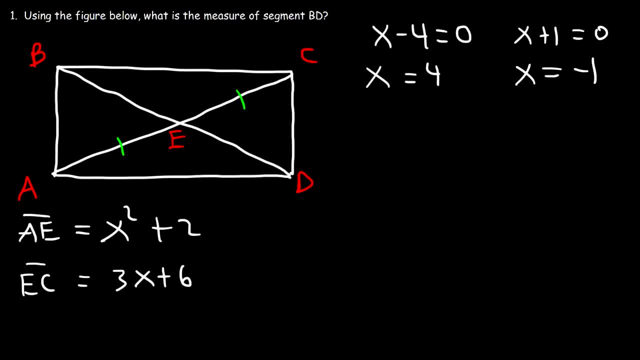 positive result, so x can be both answers. now, if x is equal to 4, ae is going to be 4 squared plus 2, which is 4 squared is 16. 16 plus 2 is 18.. and 3 times 4 plus 6, that's 12 plus 6, that's also 18.. 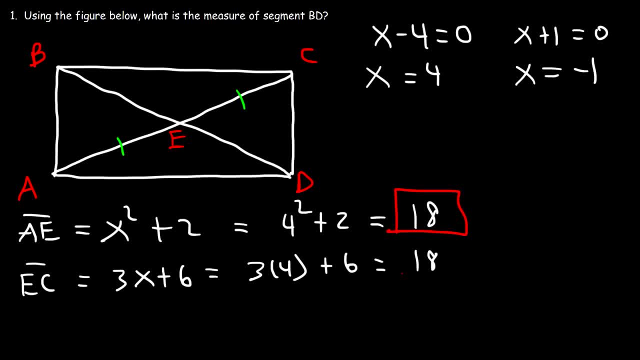 so ae and ec, potentially both 18, which means ac, the sum of ae and ec, that's going to be 18 plus 18, which is 36, and the diagonals of a rectangle are congruent, which means that ac and bd they're the same. so this diagonal is congruent to that one. 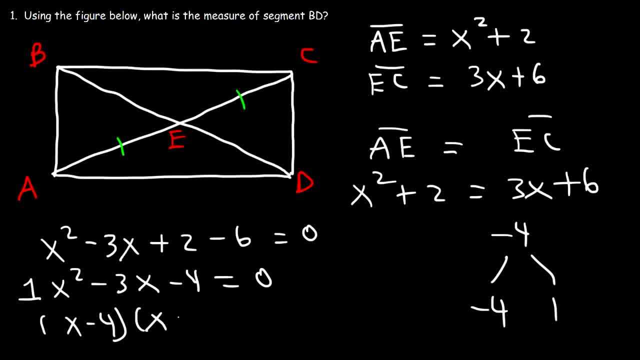 So, to factor it, it's going to be X minus 4 times X plus 1.. So now what we're going to do is we're going to take everything from the right side and move it to the left side. So what we need to do is we need to set each factor equal to 0.. 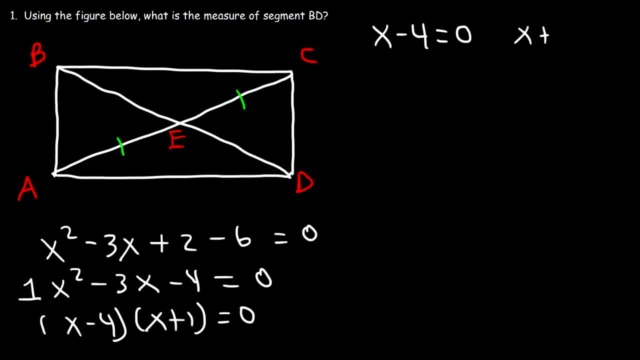 So X minus 4 is equal to 0, and X plus 1 is equal to 0. So X has to equal 4 and negative 1.. Now let's keep in mind that AE is X squared plus 2.. Because X is squared, we won't get a negative result for AE for using either of these two answers. 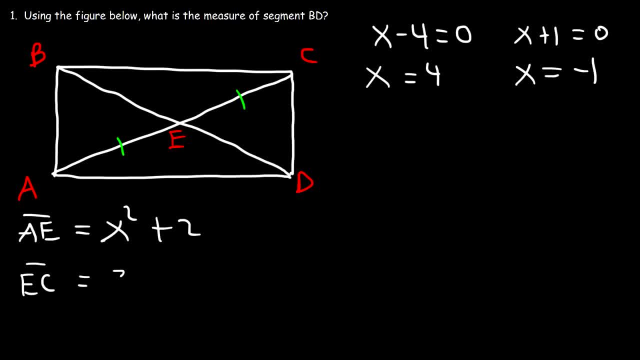 Now for EC. EC is 3X plus 6.. So if we plug in negative 1, it will still give us a positive result. So X can be both answers. Now, if X is equal to 4, AE is going to be 4 squared plus 2, which is 4 squared is 16.. 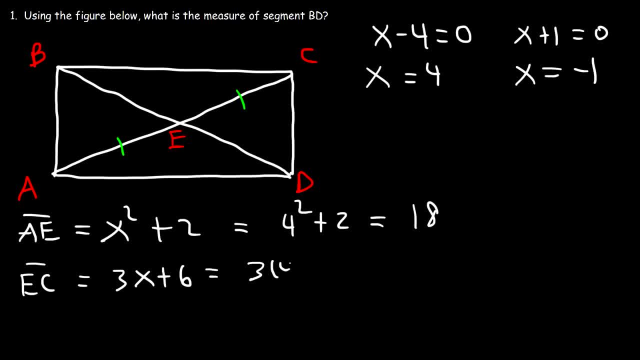 16 plus 2 is 4. squared 6 plus 2 is 18.. And 3 times 4 plus 6, that's 12 plus 6, that's also 18.. So AE and EC potentially are both 18.. 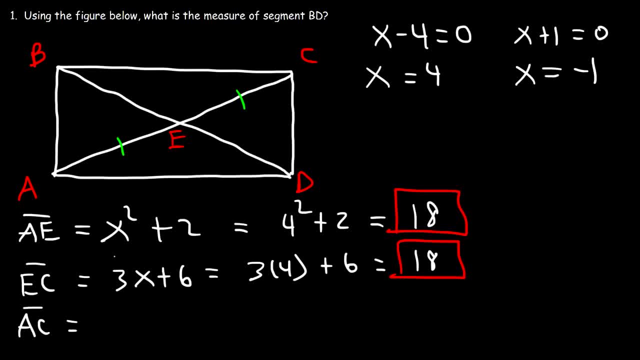 Which means AC, the sum of AE and EC, that's going to be 18 plus 18, which is 36.. And the diagonals of a rectangle are congruent, Which means that AC and MEC And BD they're the same. 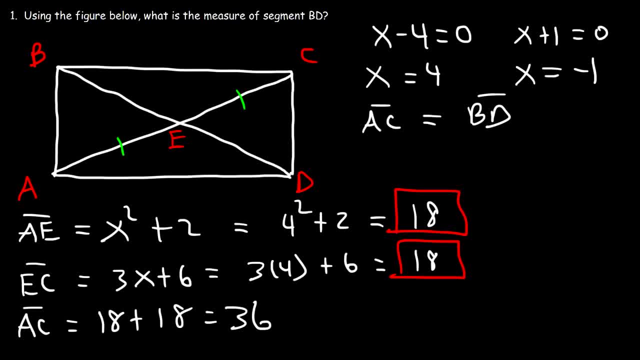 So this diagonal is congruent to that one, Which means BD is 36.. So that's one answer for BD, which is what we're looking for. Now. to find the other answer, let's use a different X value. So let's start with X. 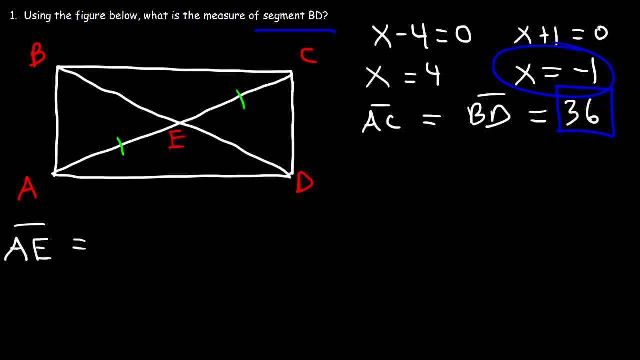 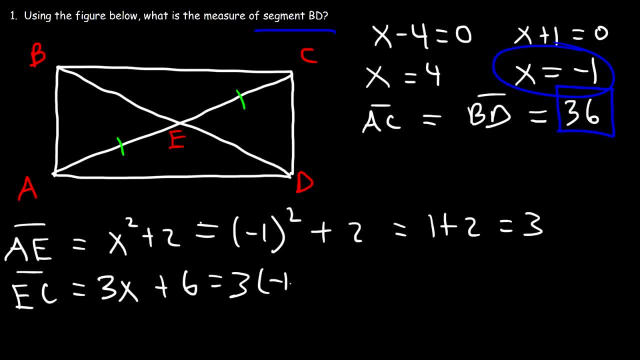 3x plus 6,, so that's going to be 3 times negative. 1 plus 6,, which is negative, 3 plus 6, and so that's 3 as well. Now AC: well, first let's start with BD. BD is equal to AC and AC is. 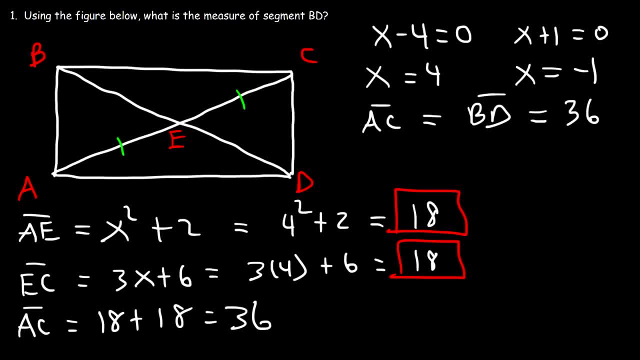 which means bd is 36.. so that's one answer for bd, which is what we're looking for now. to find the other answer, let's use a different x value. so let's start with ae. ae is still x squared plus 2.. so let's replace x with. 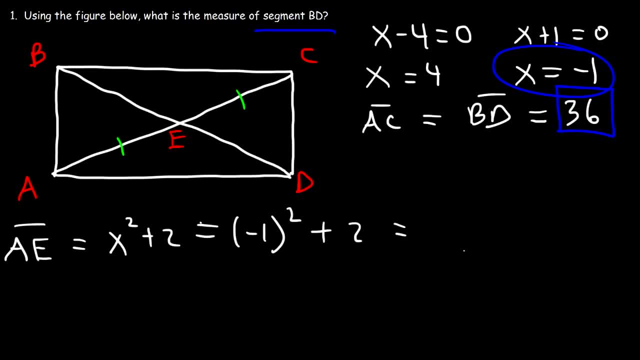 negative: 1.. negative 1 squared is 1, so it's 1 plus 2, which gives us 3.. and ec should give us the same result: it's 3x plus 6, so that's going to be 3 times negative, 1 plus 6, which is negative. 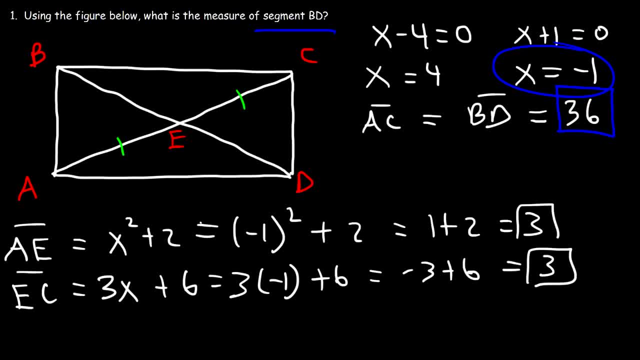 3 plus 6, and so that's 3 as well. now ac: well, first let's start with bd. bd is equal to ac, And AC is the sum of AE plus EC, So that's going to be 3 plus 3, which is 6.. 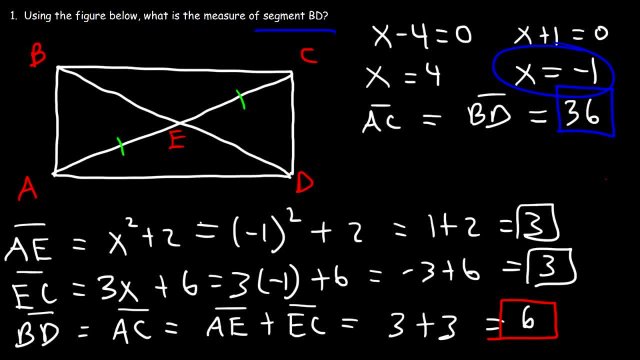 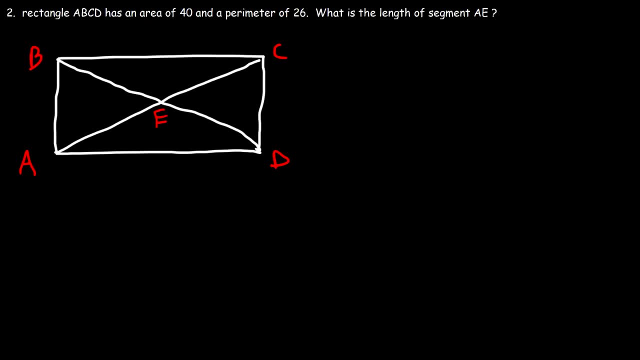 So we have two potential answers for BD. It could equal 36 or 6 in this problem, based on the expressions of AE and EC. Number 2.. Number 3.: Rectangle ABCD has an area of 40 and a perimeter of 26.. 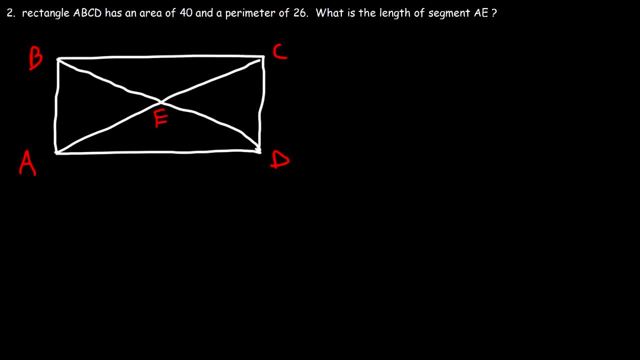 What is the length of segment AE? So for those of you who want to try this problem, feel free to pause the video and work it out. So how can we use the area and the perimeter of this rectangle in order to determine the measure of AE? 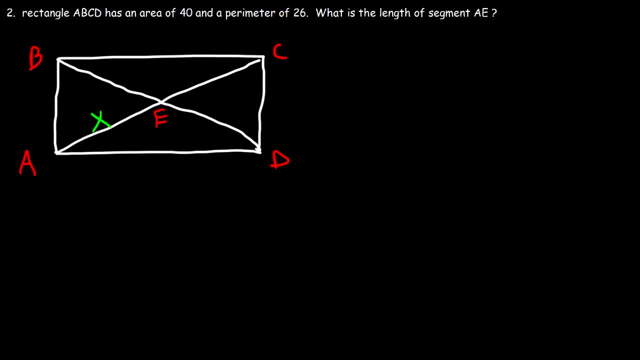 So let's call this X. How can we determine the value of X? What do you recommend that we do? Well, let's say that AD is the length and DC is the width. AC is the length of the diagonal. We said that the diagonal D is equal to well, D squared is going to be L squared plus W squared. 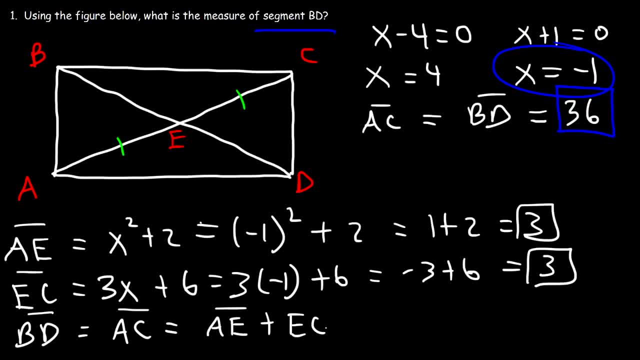 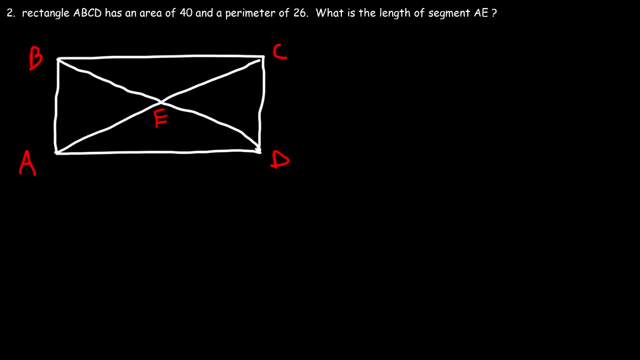 the sum of AE plus EC. So that's going to be 3 plus 3, which is 6.. So we have two potential answers for BD. It could equal 36 or 6 in this problem, based on the expression of AE and EC Number 2.. Rectangle ABCD has an area of 40 and a perimeter of 26.. What 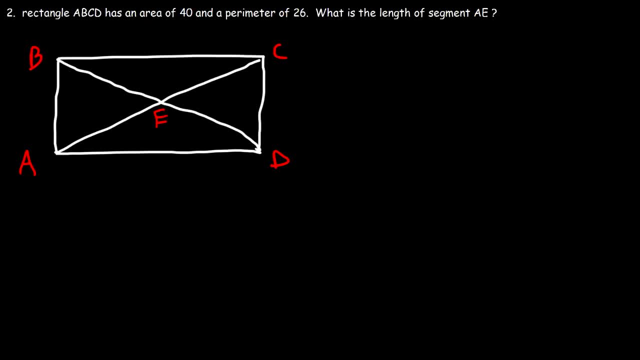 is the length of segment AE. So for those of you who want to try this problem, feel free to pause the video and work it out. So how can we use the area and the perimeter of this rectangle in order to determine the measure of AE? So let's start with BD. So, 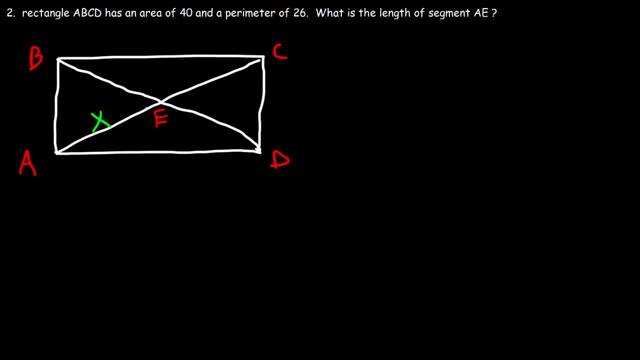 let's call this X. How can we determine the value of X? What do you recommend that we do? Well, let's say that AD is the length and DC is the width. AC is the length of the diagonal. We said that the diagonal D is equal to well, D squared is going to be L squared. 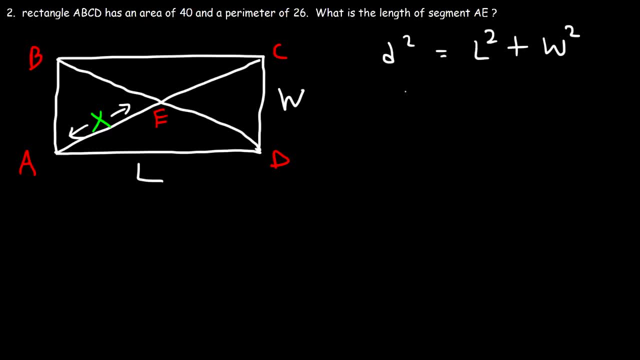 plus W squared. Now, if we could find D, which is the length of AC, AE is half of that. So AE is simply one half of AC and AC is basically the diagonal. So if we can calculate D, we can easily find AE. And in order to find D we need to determine the length and the width. 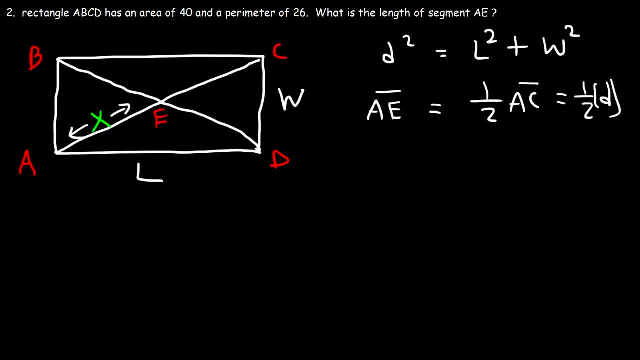 of the rectangle. So how can we do that? How can we determine the length and the width, given the area and the perimeter? Well, we need to write a system of equations. The area is the length times the width. That's like the sum of the square root squared plus E. squared. Here are some equations for purple. It says: for purple, we divide the space between the area and the width. He says: if x equals均, then that equals49 parentheses. TIMEümü squared minus the length times the width. He also says: if we define pet Standards, it's 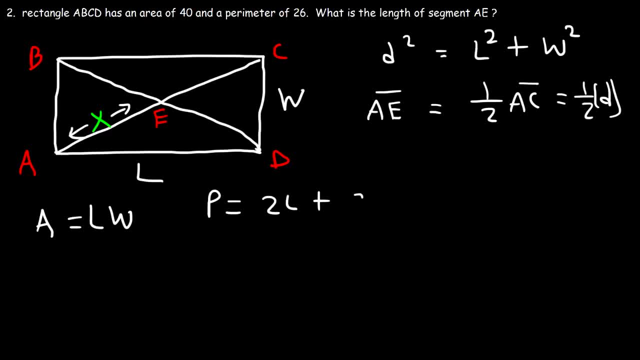 the width and the perimeter is 2L plus 2W. So we could say that 40,, which is the area, is LW and the perimeter is 26,. that's equal to 2L plus 2W. So what we're? 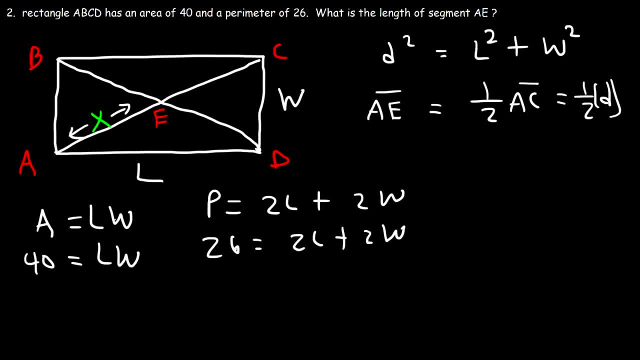 going to do is we're going to solve by substitution. In this equation let's isolate W, So let's divide both sides by L, So 40 over L is equal to W. and in the second equation let's replace W with 40 divided by L, So 26 is equal to 2L. 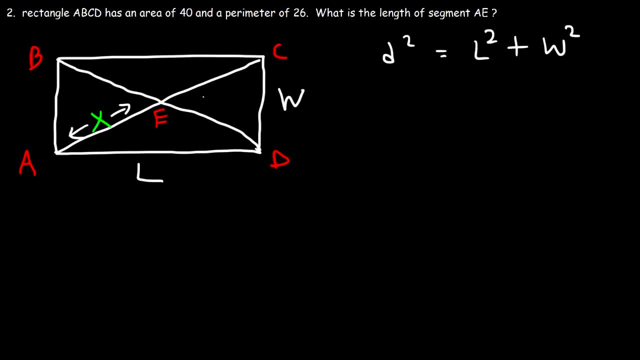 Now, if we could find D, which is the length of AC, AE is half of that, So AE is simply one half of AC and AC is basically the diagonal. So if we can calculate D, we can easily find AE. 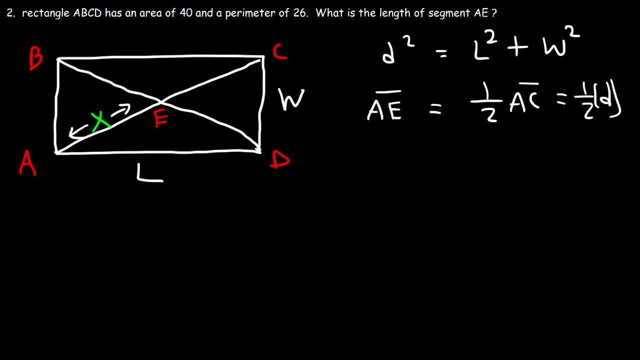 And in order to find D, we need to determine the length and the width of the rectangle. So how can we do that? How can we determine the length and the width, given the area and the perimeter? Well, we need to write a system of equations. 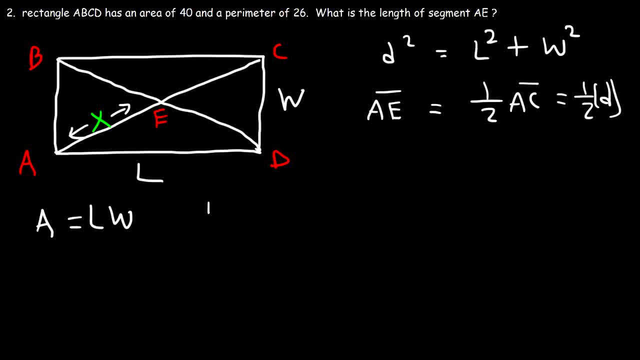 The area is the length times the width, and the perimeter is 2L plus 2W. So we could say that 40,, which is the area, is LW and the perimeter is 26.. That's equal to 2L plus 2W. 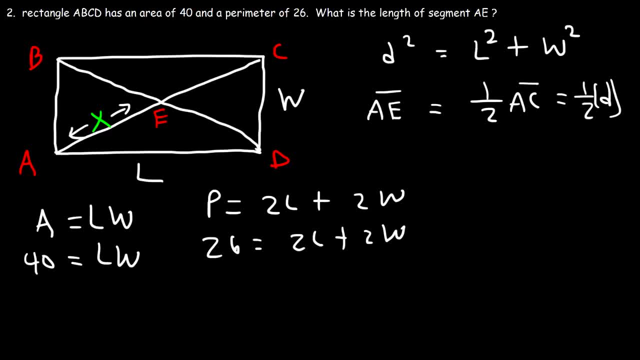 So what we're going to do is we're going to solve by substitution. In this equation let's isolate W, So let's divide both sides by L, So 40 over L is equal to W. And in the second equation let's replace W with 40 divided by L. 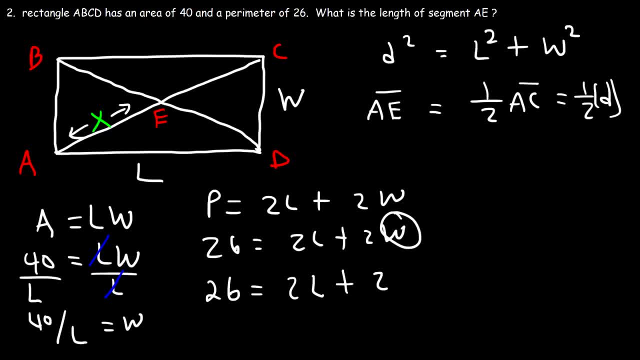 So 26 is equal to 2L Plus 2 times 40 over L. Now to get rid of the fraction, let's multiply every term by L, So this one, I'm just going to get rid of this. So this is going to equal 26L. 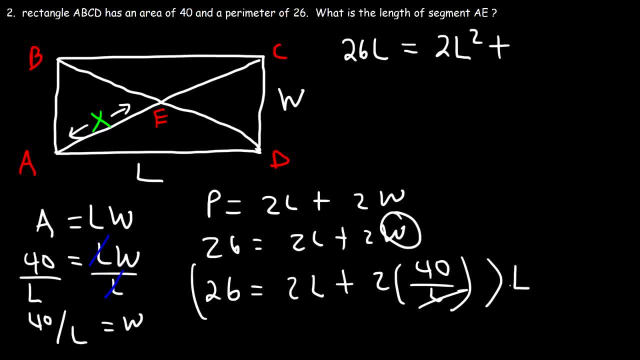 And that's equal to 2L squared. And over here the L's will cancel And we'll just have 2 times 40, which is 80.. Now let's divide everything by 2.. 26 divided by 2 is 13.. 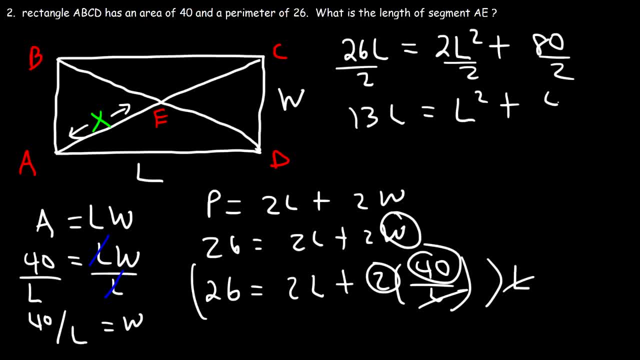 2 over 2 is 1. And 80 divided by 2 is 40.. Now let's take this term and move it to the right side. So this is going to be: 0 is equal to L squared minus 13L plus 40.. 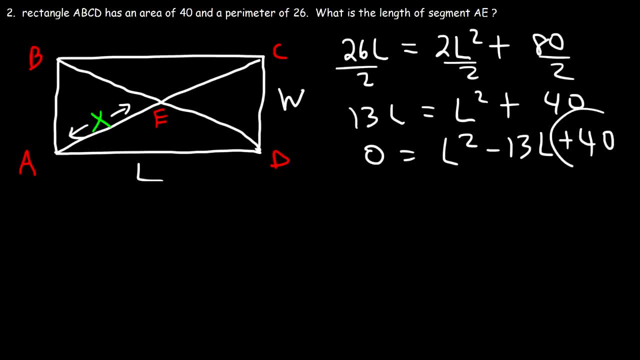 Now we need to factor the expression: What two numbers multiply to 40 but add to negative 40? 13. 5 and 8 multiplies to 40. But we need to use negative 5 and negative 8. Because those two numbers add up to negative 13.. 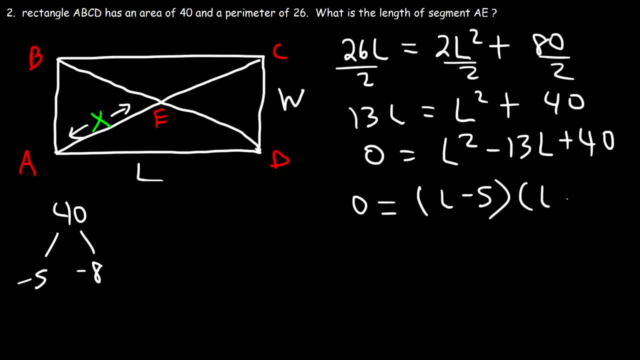 So to factor, it's going to be L minus 5 times L minus 8.. So we have two potential answers: L could be 5 or L could be 8.. Now the area has to be 40. So 40 is equal to L times W. 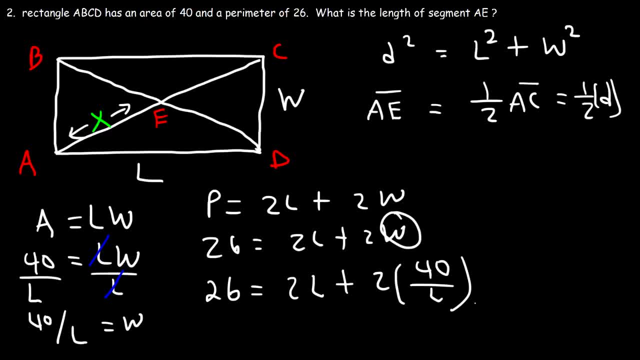 plus 2 times 40 over L. Now to get rid of the fraction, let's multiply every term by L. So this point, I'm just going to get rid of this. So this is going to equal 26 L and that's equal to 2L squared. 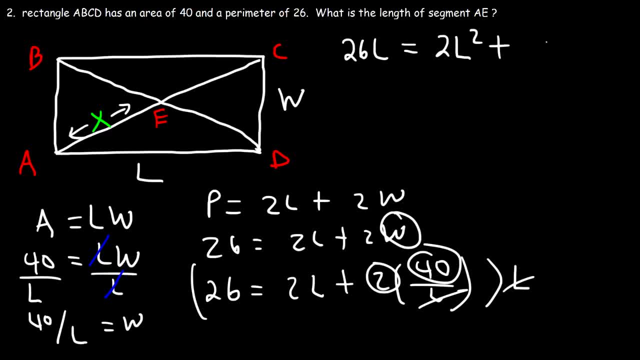 and over here here, the L's will cancel and we'll just have 2 times 40, which is 80.. Now let's divide everything by 2.. 26 divided by 2 is 13,, 2 over 2 is 1, and 80 divided by 2 is 40.. 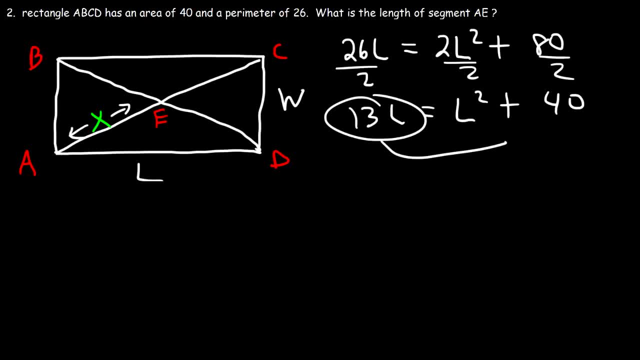 Now let's take this term, move it to the right side. So this is going to be: 0 is equal to L squared minus 13L plus 40.. Now we need to factor the expression: What two numbers multiply to 40, but add to negative 13? 5 and 8 multiplies to 40, but we need to use negative 5 and negative 8. 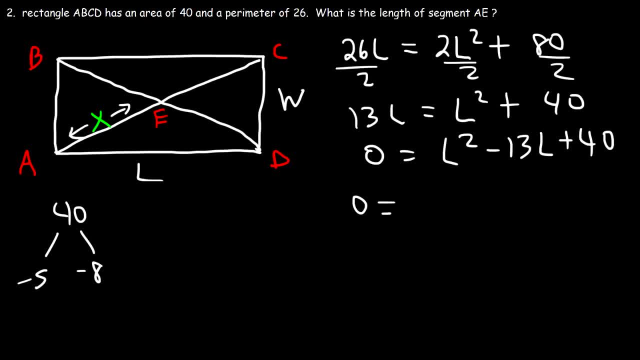 because those two numbers add up to negative 13. So to factor, it's going to be L minus 5 times L minus 8.. So we have two potential answers: L could be 5 or L could be 8.. Now the area has to be 40. So 40 is equal to L times W. 5 times 8 is 40. So if L is 5, W is 8 and 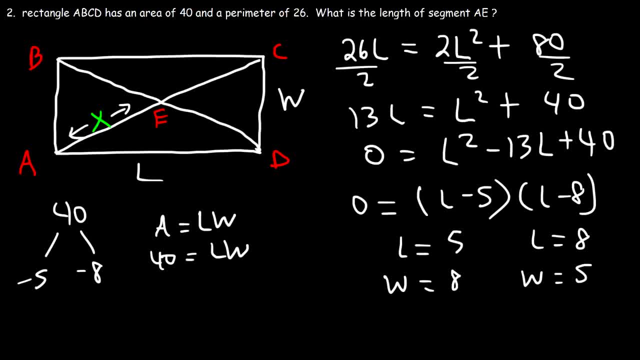 when L is 8, W is 5.. So, regardless if you choose this answer or this answer, the left of the diagonal will still be the same and AE will still be the same. So we could just choose one of those two answers. So we're going to say that L is 8 because it appears to be 8.. So we're going to 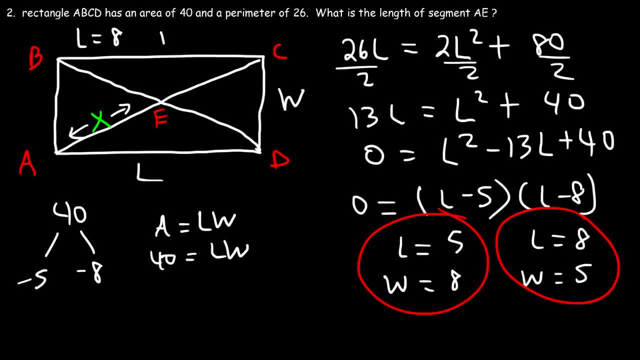 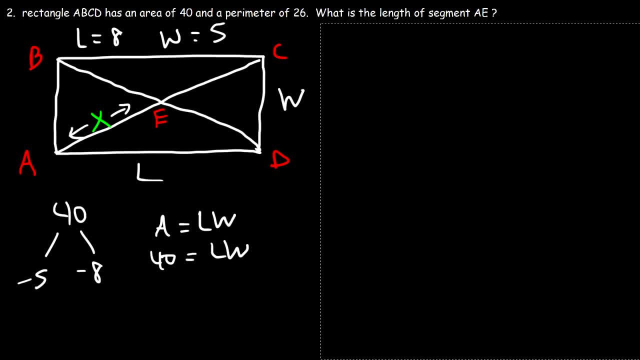 say that L appears to be longer if you look at the shape of this figure, And W, which appears to be the shortest side, we're going to say it's 5.. So D squared is L squared plus W squared, L is 8, W is 5.. 8 squared is 64 and 5 times 5 is 25..